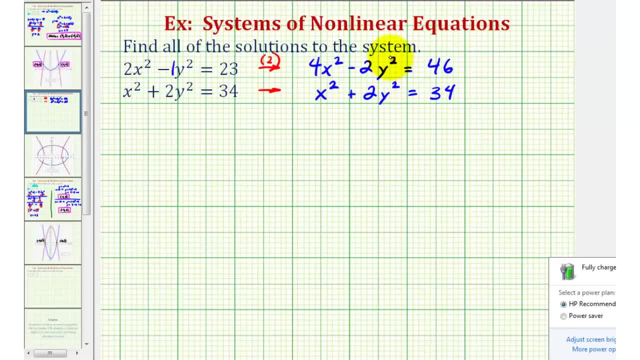 meaning both of them are y squared. in this case, If one was y and one was y squared, we would not be able to eliminate the y terms. So now we'll add these two equations together. Notice, when we do this, the y squared terms are opposites, so they'll add to 0.. 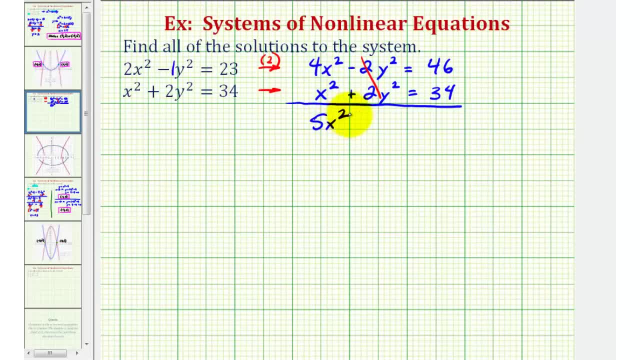 So we'll have: 5x squared equals 46 plus 34 is equal to 80.. To solve this for x, we'll first divide by 5 on both sides. So we have x squared equals 80, divided by 5 is equal to 16.. 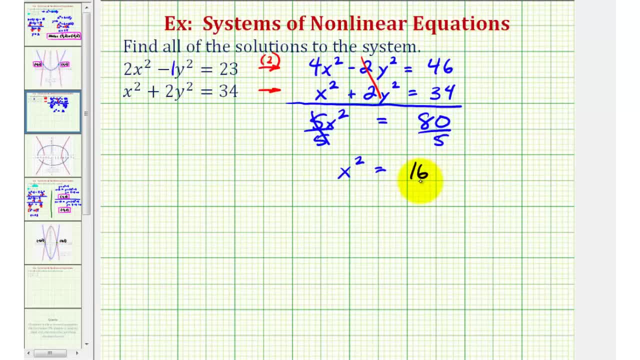 At this point we should recognize we'll have two values of x that satisfy this equation. Since we have x squared and we want x, we'll take the square root of both sides of the equation and we'll include a plus or minus sign here to make sure we obtain both solutions. 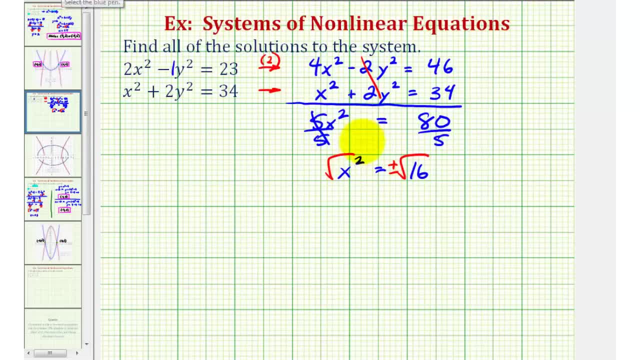 So the square root of x squared equals 4y squared minus 4y squared. We'll take the square root of both sides of the equation and we'll include a plus or minus sign here to make sure we obtain both solutions. So the square root of x squared is equal to x. 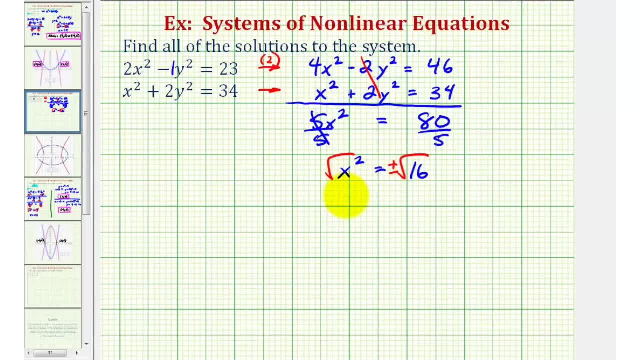 It's actually the absolute value of x, Another reason why we have two solutions. And then the square root of 16 is equal to 4.. So x equals either positive or negative 4 or plus or minus 4.. And now to find the corresponding values of y. 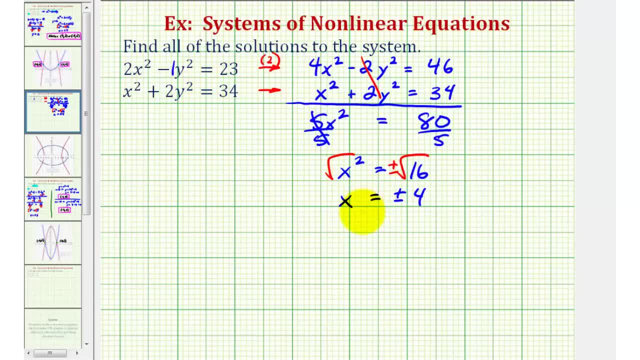 that give us the solutions for the system. we'll perform back substitution. Let's go ahead and use the first equation here to find the corresponding values of y. So if we use the equation, 2x squared minus y squared equals 23.. Let's first solve this for y squared. 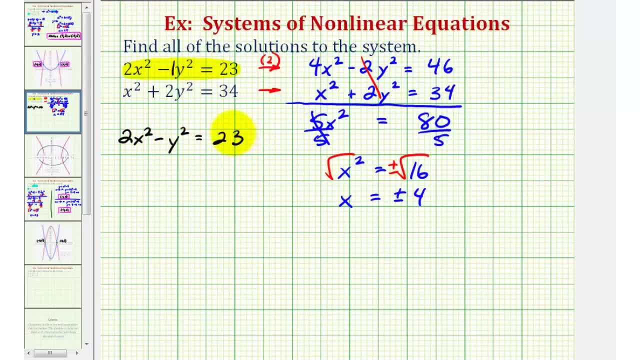 So we're actually going to add y squared to both sides and subtract 23 on both sides. That would give us 2x squared minus 23 equals y squared. Let's go ahead and switch this around: We have y squared equals 2x squared minus 23.. 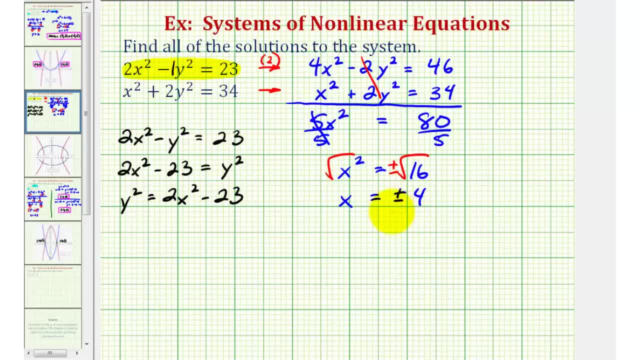 Now we know that x can be either positive 4 or negative 4.. Let's substitute x equals positive 4 first to find the corresponding values of y. So we would have y squared equals 2 times 4 squared minus 23.. So we have y squared. 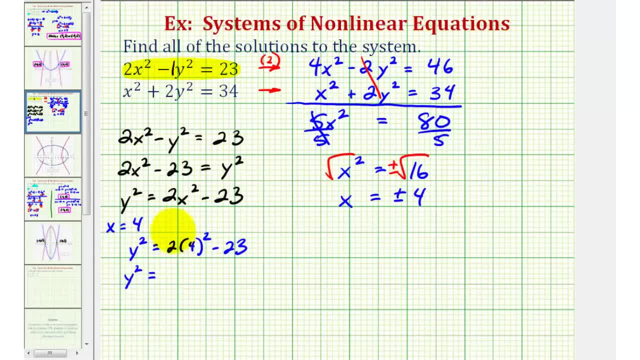 equals 4 squared is 16, 16 times 2 is equal to 32.. Well, 32 minus 23 is equal to 9.. So we have y squared equals 9.. So again to solve for y, we'll take the square root. 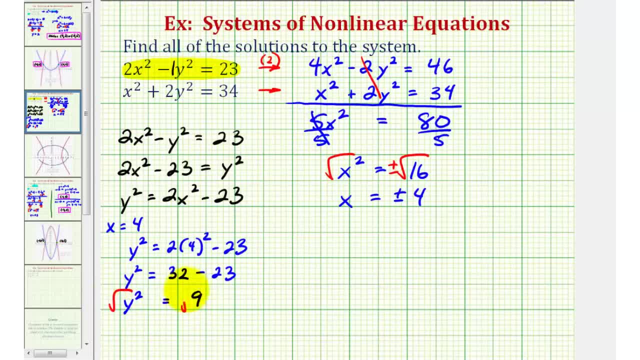 of both sides of the equation, We'll have two solutions, one positive and one negative. Since it's the square root of nine is equal to three, we'll have y equals plus or minus three. So from this outcome we know we have at least two solutions. 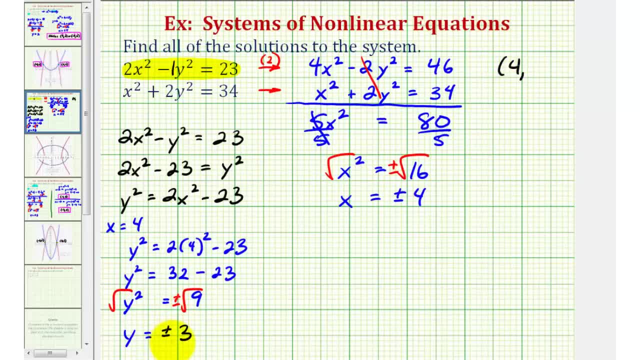 When x is positive four, y can be either positive three or negative three. So this would be one solution. The second solution would be four negative three. Remember, when giving the solution as ordered pairs, the first coordinate is always the x coordinate or x value. 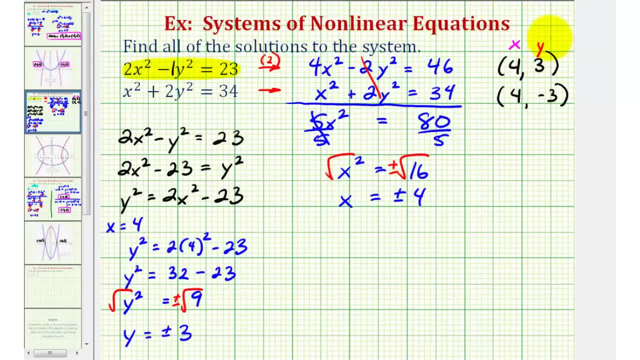 and the second coordinate is the y coordinate or y value. Remember we also said that x can be negative four. So, using this equation again, we'll substitute negative four for x, So we would have: y squared equals two times negative four squared. 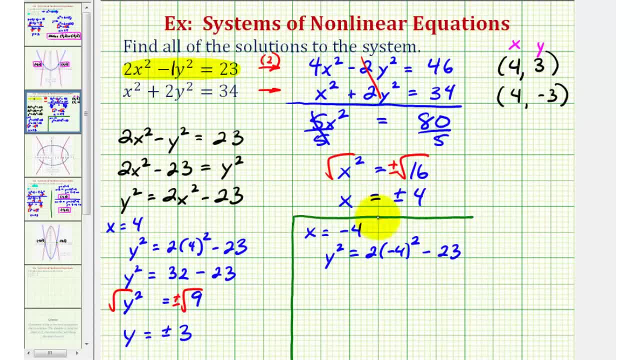 Negative four squared minus 23.. Well, negative four squared is equal to positive four squared. So if we simplify this, we're going to get y squared equals nine again. So if we take the square root of both sides of the equation again, we'll have y equals plus or minus three. 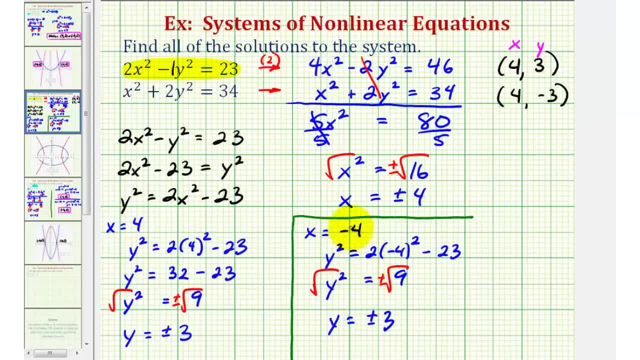 So this outcome gives us two more solutions. When x is negative four, y can be positive three or negative three. So the third solution would be negative four comma three, And the fourth solution would be negative four comma negative three. 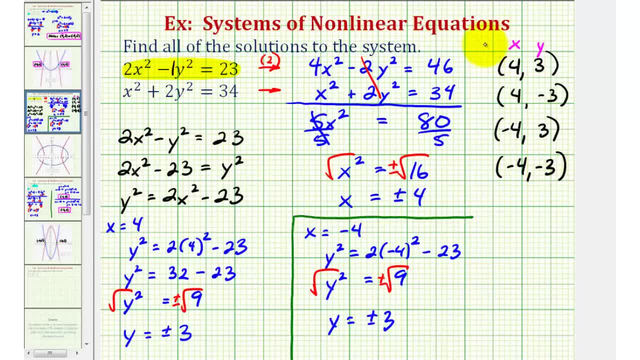 So this system actually has four solutions given by these ordered pairs And to verify this, we're going to graph both equations on the same coordinate plane and our graphs should intersect at these four points. Let's take a look. The first equation is actually a hyperbola.